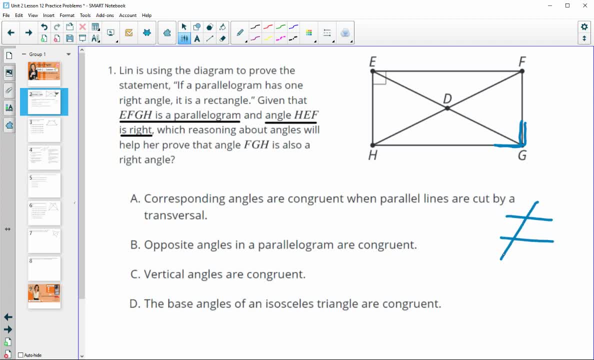 transversal, which is definitely a true statement. So if we have parallel lines, the corresponding angles are congruent, but these two angles in question are not corresponding angles, So this is not what's going to be helpful. Opposite angles in a parallelogram are congruent. 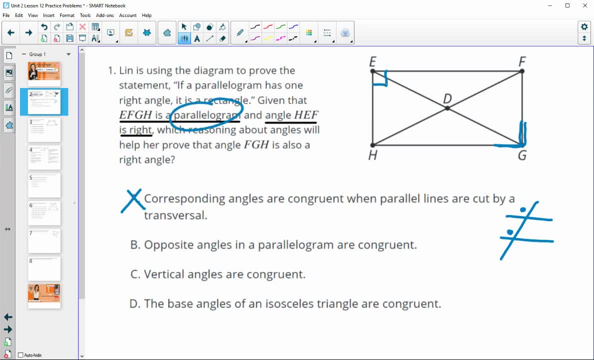 So we do definitely have a parallelogram. Okay, we know, this one's a right angle, and then this is the one across from it. And in a parallelogram, opposite angles are congruent, and so that one would be good. Vertical angles are congruent Again. 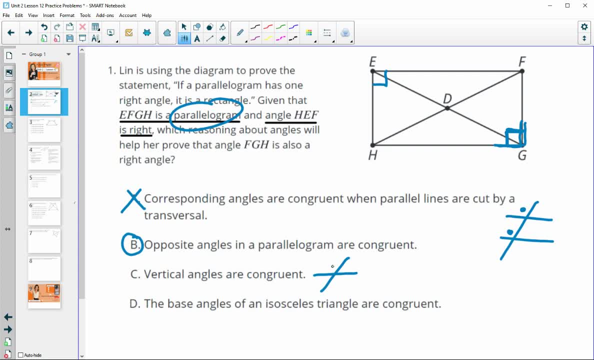 this is a true statement, just we don't have vertical angles here. Vertical angles are right next to each other or, sorry, right across from each other, like this, So that doesn't work. And then base angles of an isosceles triangle are congruent is a true statement, but not what we. 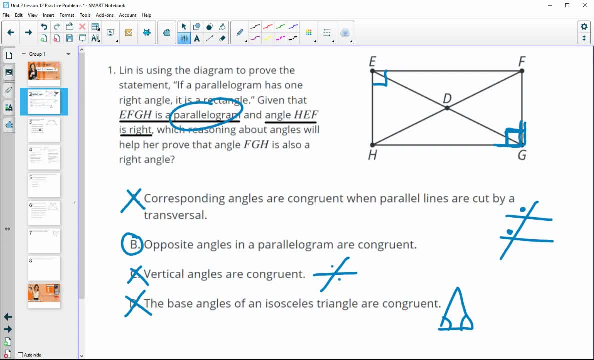 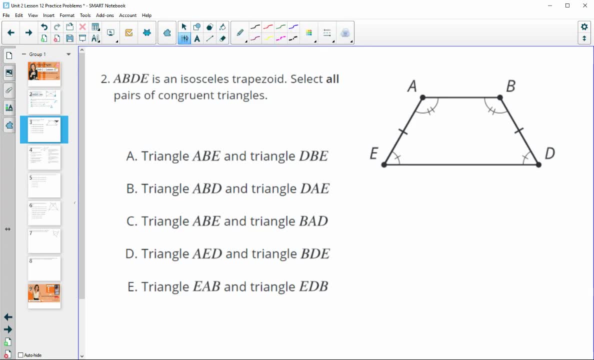 have in this diagram All right. number two says ABDE is an isosceles, trapezoid, Select all pairs of congruent triangles. So letter A says triangle ABE, So ABE. And let's just mark up what we have here as we draw the triangle. So we know. 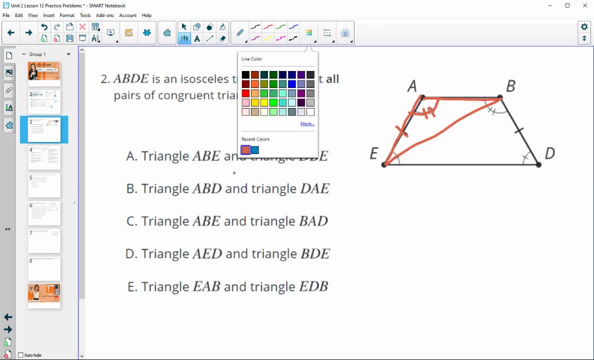 this angle, we know this side, and then this is kind of cut so we won't mark anything there. It's congruent to triangle DBE And so we've got this angle and we've got this side and then they share this side. Now, the way that they did this, they have angle A first. 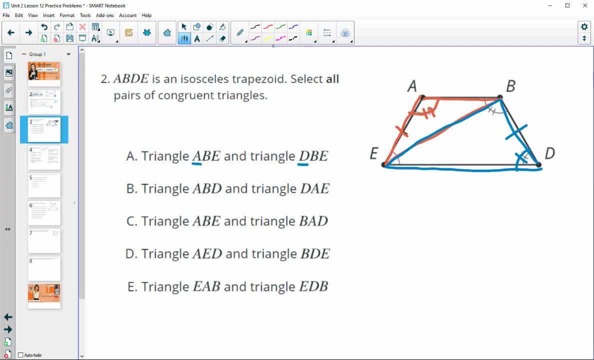 angle D first. Well, angle D and angle A are not the same size angles, So these two triangles are not congruent. Letter B says triangle ABD. Is that one congruent to DAE? And so this one again. they marked up this little angle A with this angle D which has a potential. 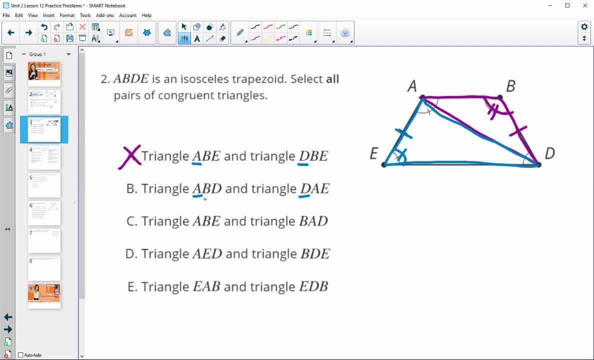 to be the same. So let's look at some of the other stuff: B with this, B angle here with A here, and those are not the same. So this is not true. And you could also look at D with E not being the same and they don't have the same. 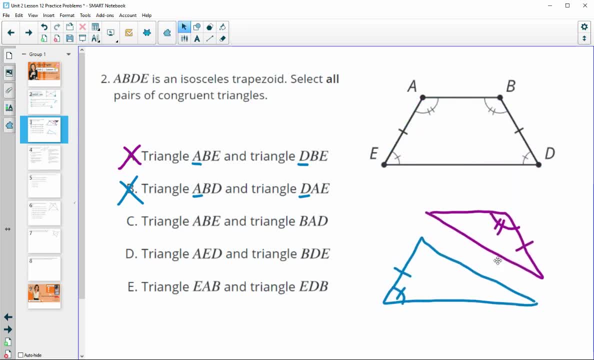 Side lengths either. So if we like kind of pulled this off, you could see these that they don't have the same kind of angles marked there. They do have the same side. They shared this side right. So we've got two sides and an angle and this is two sides and a different angle, So they don't. 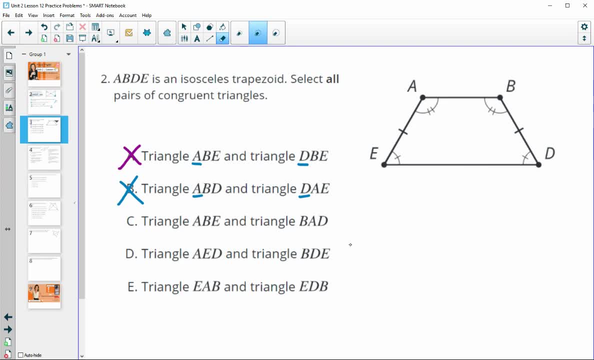 have the same congruent angle marked. So that's not going to prove that they're congruent either. Triangle, ABE: So we've got this angle in the purple one and then that side. So let's pull these two off and take a look at them. 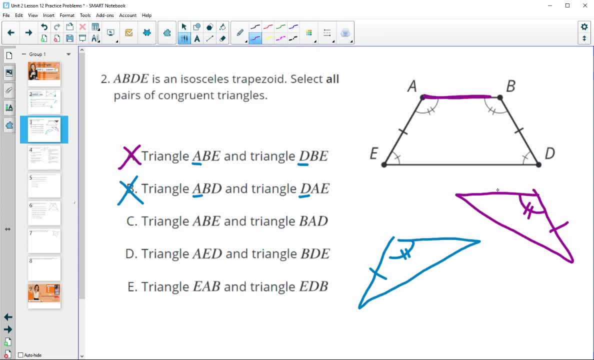 And they also shared a side, So they shared this side in both. So we've got this side congruent to this side. So now we see on these two pictures that we've got two sets of sides And the angle between them marked as congruent and that is side angle side. So these two triangles are congruent. 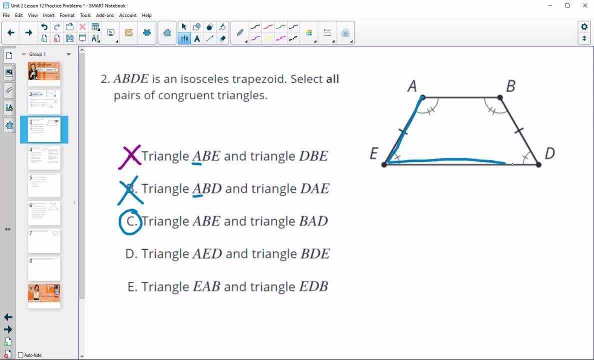 D has us looking at triangle AED And then triangle BDE, And now these share this bottom side. So let me mark that when we pull it down, And then let's mark it on this one, now that we know that it was shared. 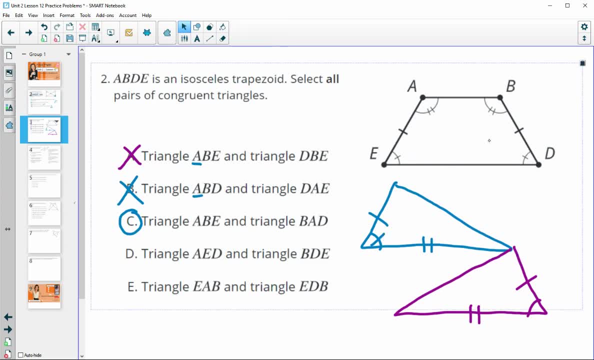 Okay. So again we've got two sides and the angle between them marked as congruent. So these two triangles are congruent by side angle side. Then let's just make sure that they followed the correct order. So these two triangles are congruent in the way that they marked them. 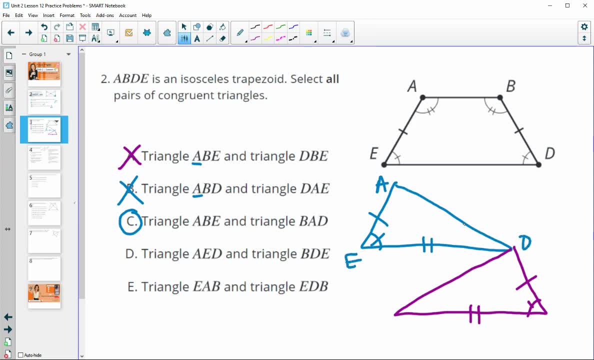 So we had AED and then this was EBD. So let's set them. Let's see what order we went. So we went AED, so we went down the one tick mark to the two tick mark. Then this one was BDE, same order. 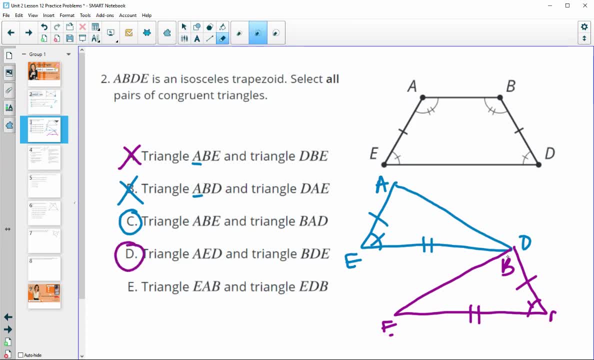 So these two triangles are congruent. Then E has us looking at triangle EAB and then also EDB And we can see that those are not going to be congruent. They've got a different angle with the side, So this one has the one tick mark angle and this one had the two tick mark angle. And then they're also just congruent. So this one has the one tick mark angle and this one had the two tick mark angle. So this one has the one tick mark angle and this one had the two tick mark angle. So this one has the one tick mark angle and this one had the two tick mark angle. 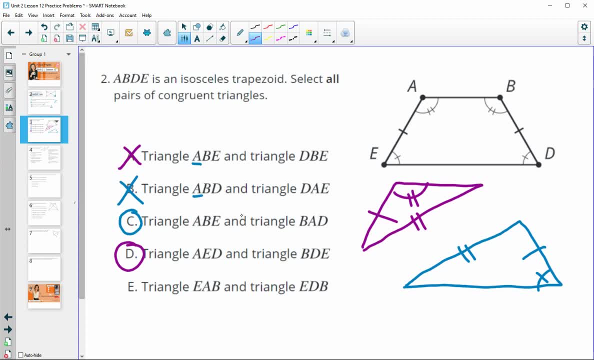 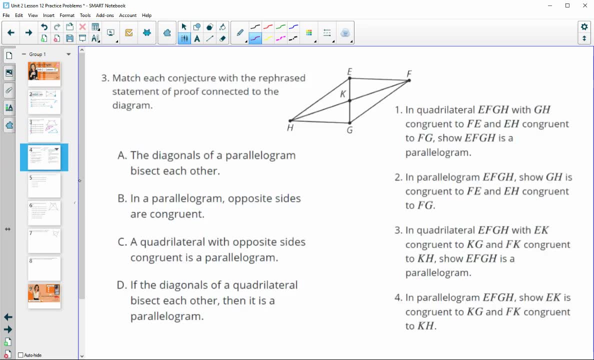 So just sharing two congruent sides and the angle, not between, even though the angle isn't congruent anyway. So this one would be false. Number three match the conjecture with a rephrased statement of proof. So we're looking at restating this conjecture in what we would need to be proving. 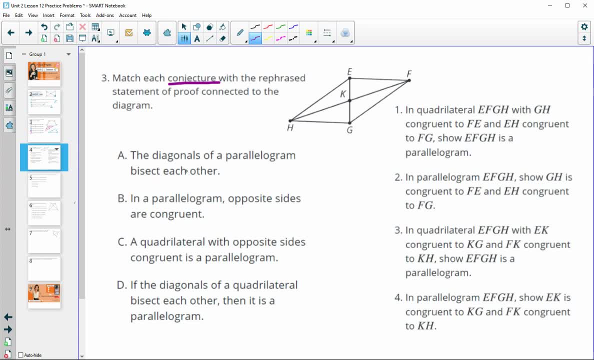 So A says the diagonals of a parallelogram bisect each other. So we're going to be looking at having talked about about a parallelogram first and then proving that these little segments here are congruent, since that's what bisect means. 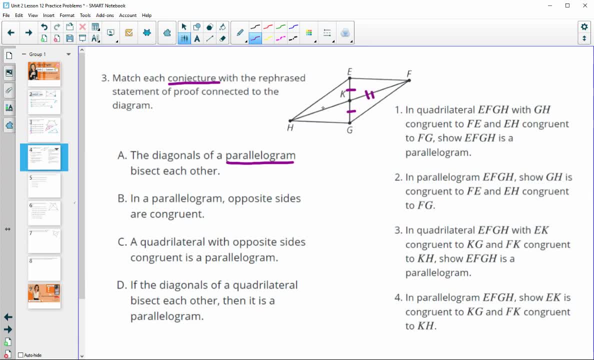 So bisect would mean that we would have this segment congruent to this one and this one congruent to this one. So let's look for in a parallelogram. So we're looking at number two and number four And then we want to be seeing where we're talking about the diagonal segments. 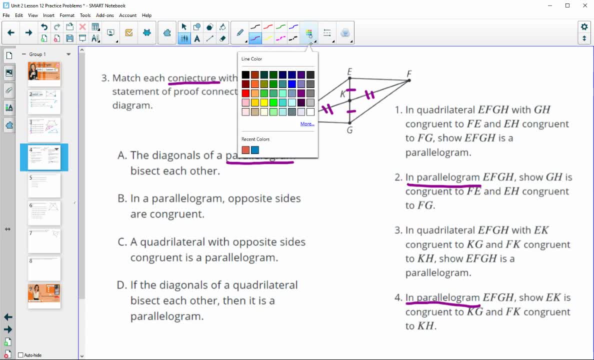 So in number two it talks about GH being congruent to EFE. So those are not the diagonals, those are opposite sides. So let's look at the next one. So number four talks about EK being congruent to KG. 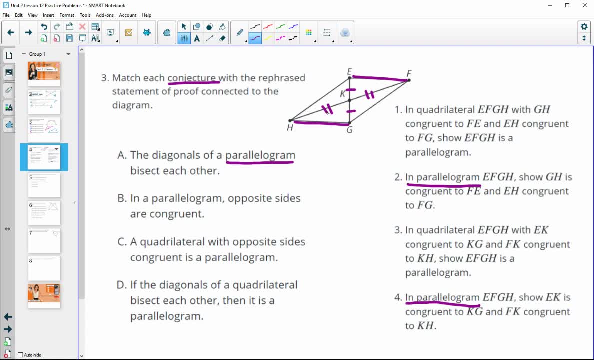 So that is the diagonal pieces and then FK congruent to KH. So we would rewrite. we would rewrite this one like number four. So then, now that we've looked at this, one says parallelogram, let's look at another one that says parallelogram. 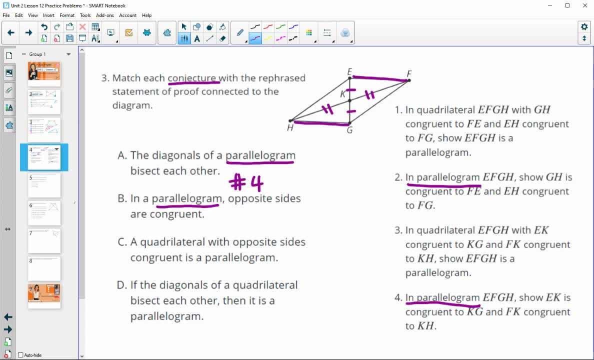 Which is B, and this one does talk about the opposite sides. So that would be said for this one that in parallelogram, EFGH, GH is congruent to FE and EH is congruent to FG, So naming those opposite sides. So that's number two. 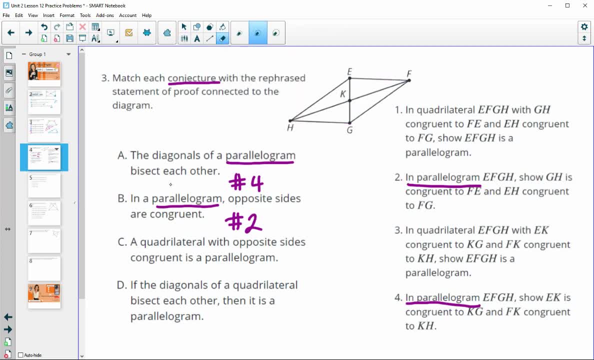 Then we can look at these next ones. talk about being a quadrilateral with opposite sides congruent. This is a parallelogram, So quadrilateral. they're going to talk about the opposite sides and then conclude that it's a parallelogram. 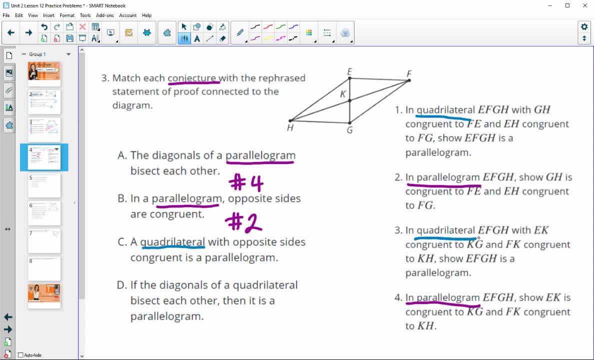 And so we know that we're looking in number one or number three, where they talk about the opposite sides first. So in quadrilateral EFGH, GH is congruent to FE. So those are. this one is talking about opposite sides. 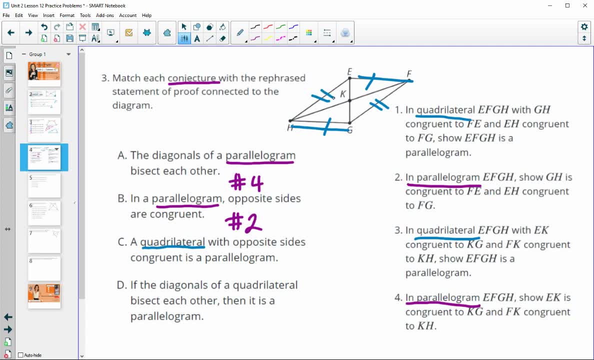 They're saying this is congruent to this and EH is congruent to FG, Then it's a parallelogram. Then we'll show that it's a parallelogram. So C is going with statement number one. So that leaves number three to go with D. 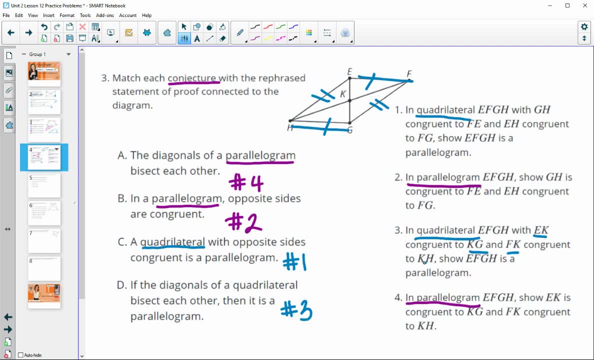 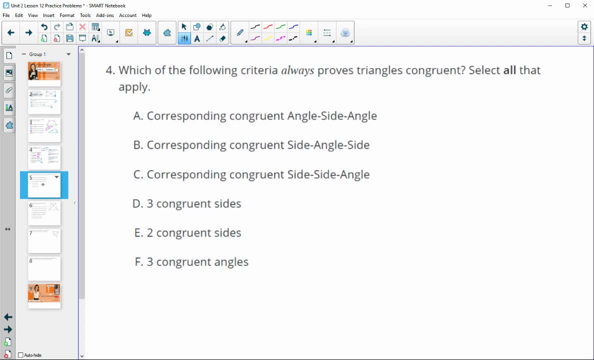 which does talk about a quadrilateral with the diagonal pieces congruent and then, concluding, it's a parallelogram. Number four, which of the following criteria always proves that triangles are congruent? Select all that apply. So, if we have corresponding congruent angles, 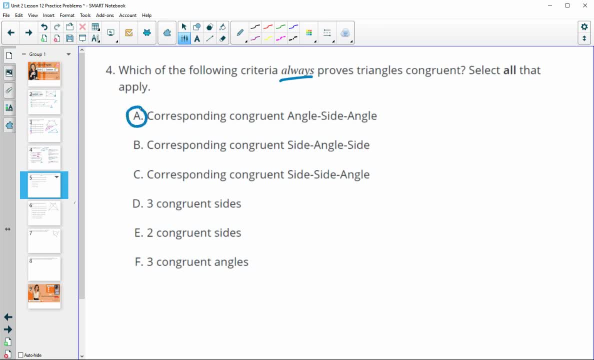 angles with a side in between. that would be true. Okay, we learned that you can have two angles in the included side. This next one says that we have two sides and the included angle. We know that that is true, Corresponding congruent, where we have two sides and the non-included angle. 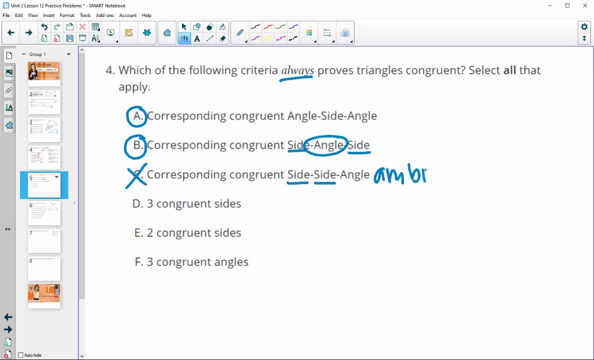 This one is false. This is that ambiguous case where there could be two triangles made with that same information, Three sets of congruent sides. definitely true. If we know two sides are two sets of sides are congruent, that is not enough. And if we know three angles are congruent. 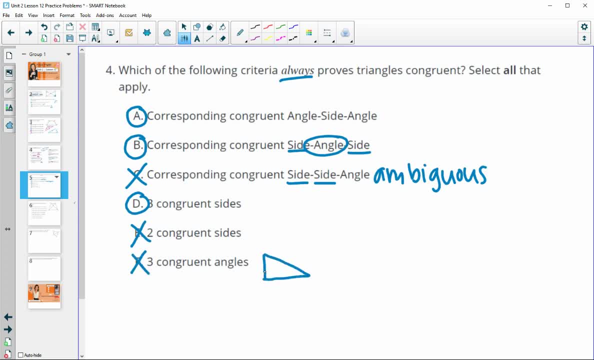 that is not enough. So, remember, we could just kind of look at this triangle and it's kind of easy to show here. I could just make this bigger. The angle stays the same size, So all of those angles are staying the same size. 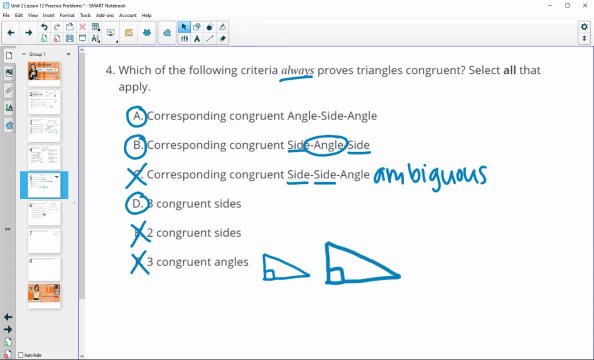 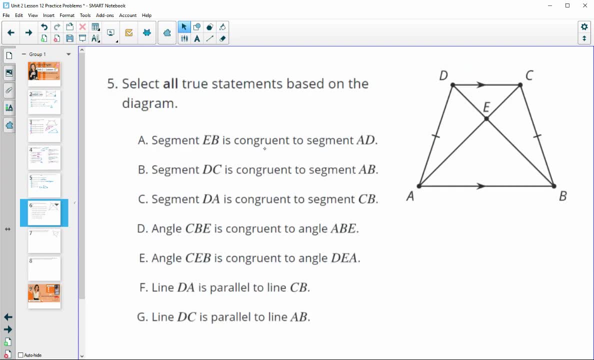 but the triangles are. they're not two different sizes, so not congruent. Number five: select all true statements based on this diagram. So segment EB: this segment is congruent to segment AD. That is not true. Segment DC is congruent to segment AB. 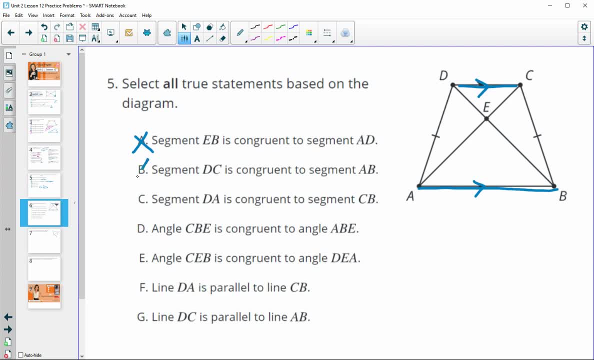 We see that it's got these arrows on it, but arrows don't mean congruent, They mean parallel. Segment DA is congruent to segment BC and we see the tick marks confirming that. So this is true. Angle CBE. 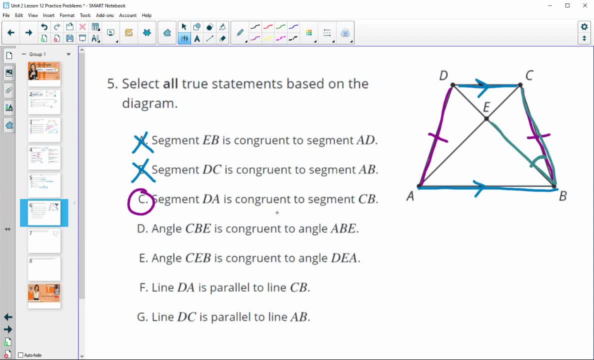 So CBE. is this one congruent to angle ABE? So are these two angles congruent? And that is false. Angle CEB, So CEB. is this one. So angle CEB congruent to angle DEA? this one. 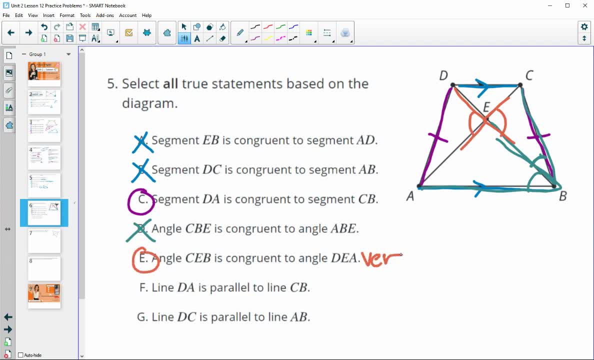 and that is true. These are vertical angles. Line DA is parallel to CB, So these purple ones here. so this is parallel to this. That is false, false. and then dc is parallel to a, b, and we know that's true because we saw those arrows on it. 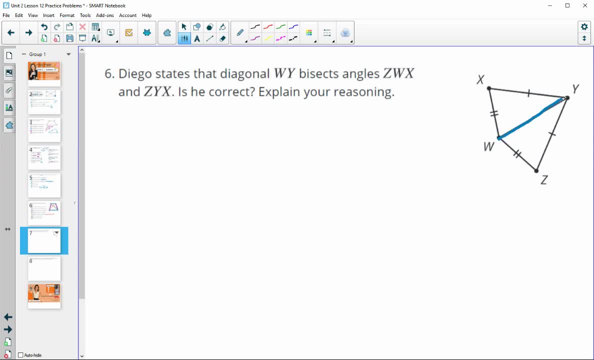 number six, diego states that w? y is the bisector of this um angle x, y, z and also x, w, z. is he correct? explain your reasoning. and so we know that. yes, he is correct, because w? y splits the kite into two congruent triangles, so the corresponding angles will be congruent, and we know that those little angles on either side. 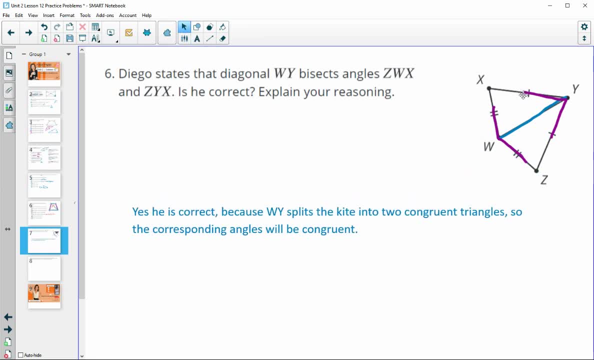 of um on either side of the diagonal here. so this one and this one are congruent. this one and this one are congruent. and if you wanted to kind of write that out- but you don't want to keep writing all of these angles- you could put little numbers in here. so you could do one. 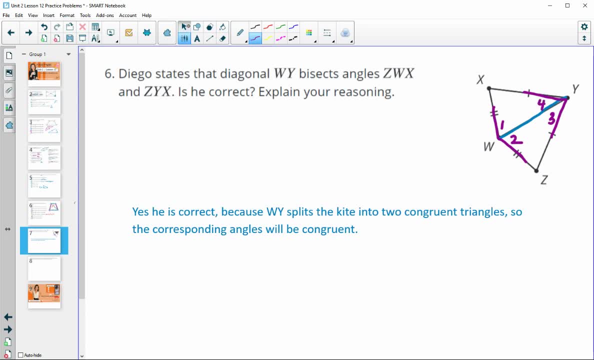 two, three, four, just to maybe make your um typing easier, your writing easier. uh, so congruent triangles, so the corresponding angles will be congruent um, meaning angle one is equal to angle two and angle three is equal to angle four. so the um larger angle w and y are both split into two congruent angles. 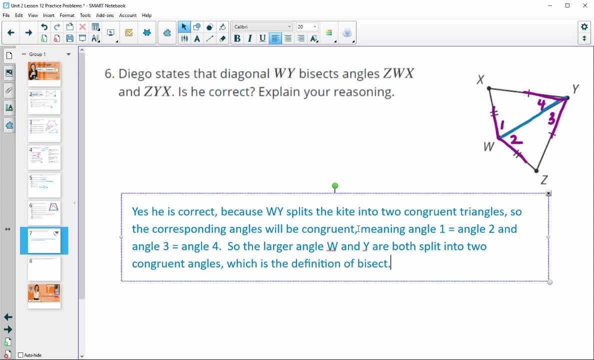 which is the definition of bisect, so something along that line. for this one. It doesn't have to be exactly that, but that these two triangles will be congruent by side, side side, since they share this side in here. So then, these two angles are going to be congruent because they're corresponding, which then, is the definition of a bisector. 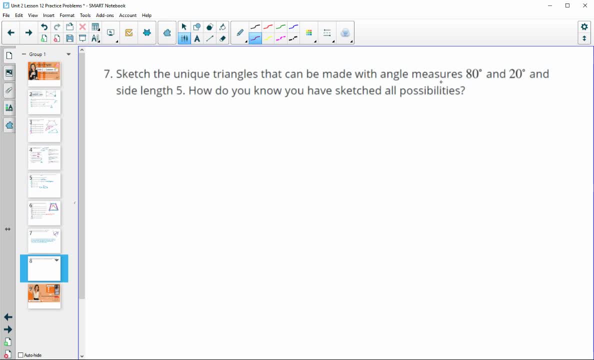 Number seven says: sketch unique triangles that can be made with the angle measures of 80,, 20, and a side length of five. How do you know? you've sketched all the possibilities. So when we see two angles, remember we can find the third one, because we know the total of all three is 180. 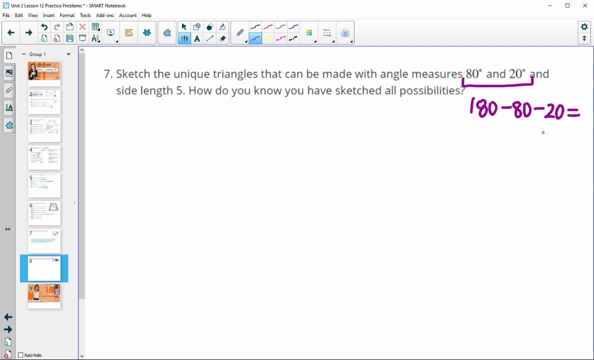 So we can subtract off 80 and 20 from 180 to get that the third angle is 80. So we now know that this triangle has two 80 degree angles, meaning it's isosceles. So the only two ways for this to work would be that.